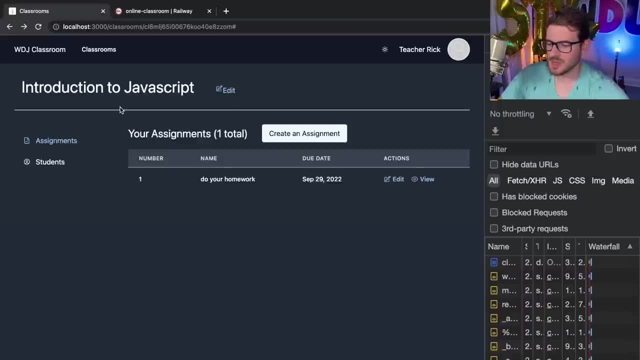 of stuff for their machines. um, so i have this uh online classroom thing i've been working on during some live streams, and in order for other people to kind of jump on and work on this project, they would have to set up their own database, right, so installing postgres on your machine, it's not. 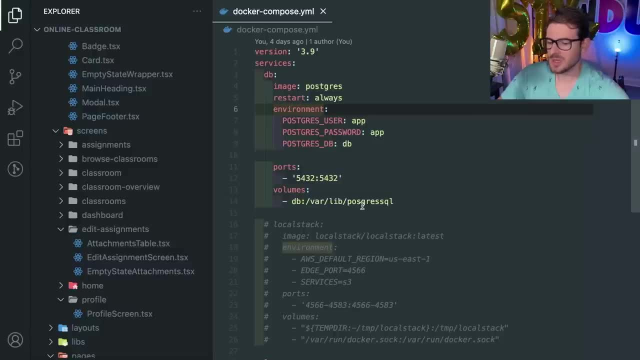 too much work, but there is a lot of potential things and snags you can run into, depending on your operating system, depending on you know the version of mac you're on, or you know just a bunch of variables that can make the experience of setting up postgres difficult, right, you might? 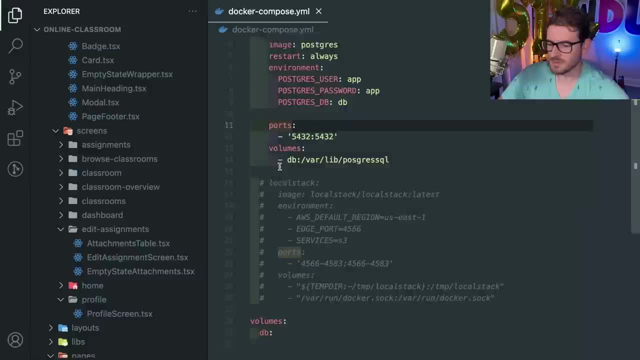 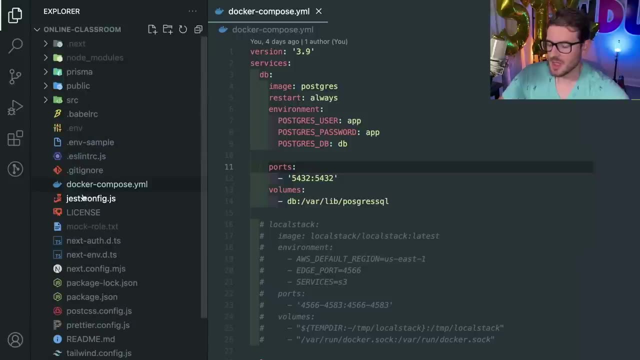 have to, like run some commands with admin access. sometimes you screw stuff up with like permissions and you have the chmod files. so this, this project here. this is an xjs project using the t3 stack, but i used a docker compose file to basically speed up the process of setting up postgres on my machine, and i was able to do that with a lot of. 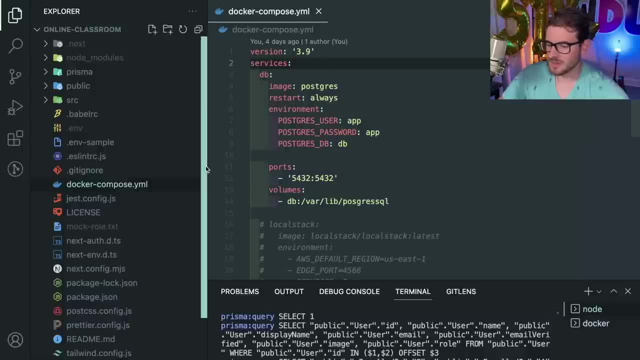 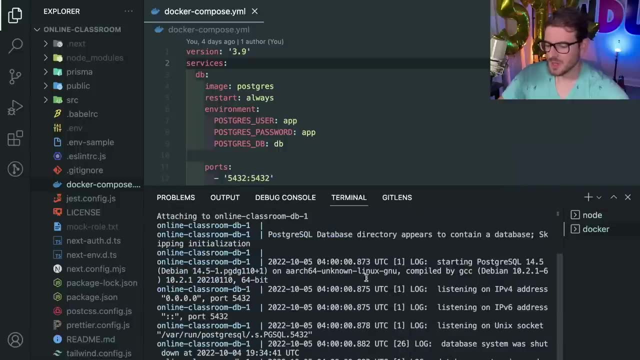 ease. so i'm going to go ahead and spin up a local postgres service, right? so if i go ahead and just show you that real quick, i have a terminal over here and the second terminal here is actual is actually running this docker compose up. so let me just kind of give you a walk through of what docker. 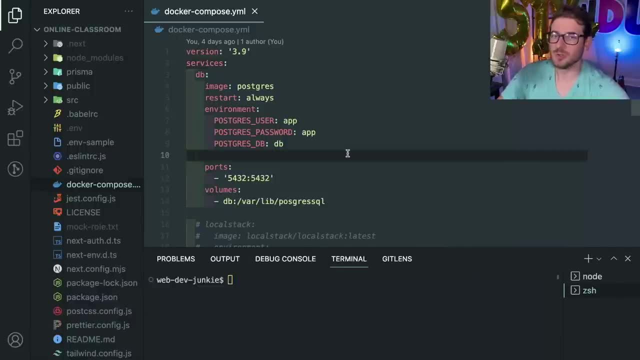 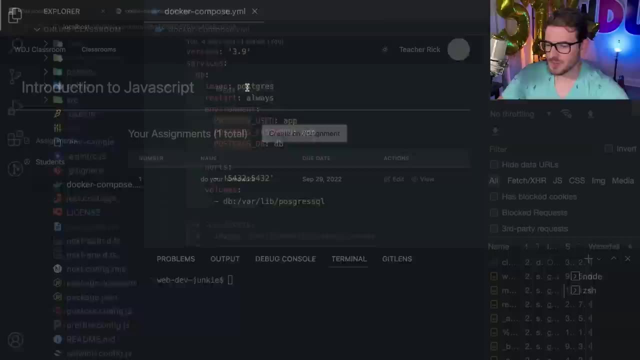 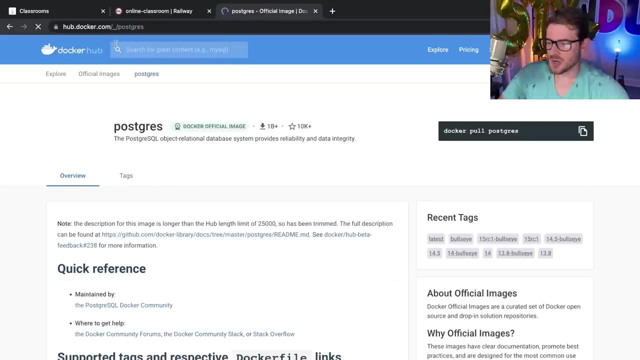 compose is and how it potentially uses docker under the hood to run this database, so you can specify the image name, which i believe if you go to like docker containers and look for this image there's, there's dockerhubcom, which actually has a bunch of images on them. 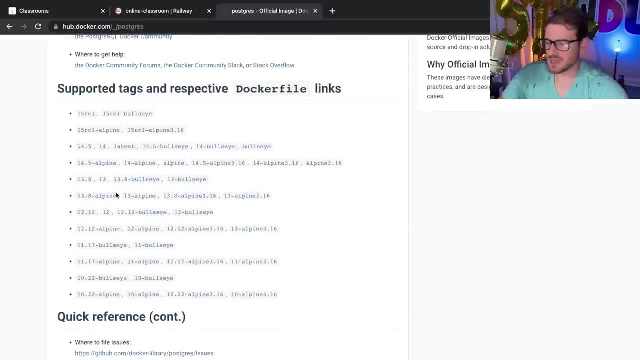 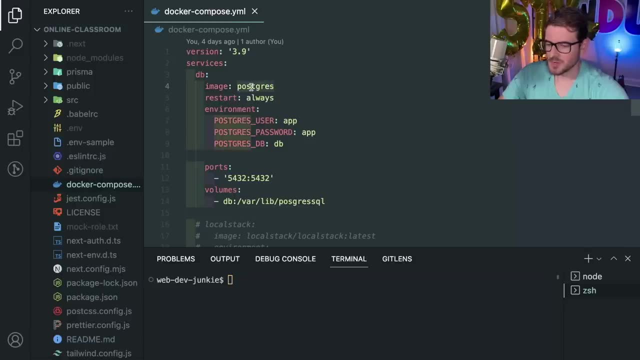 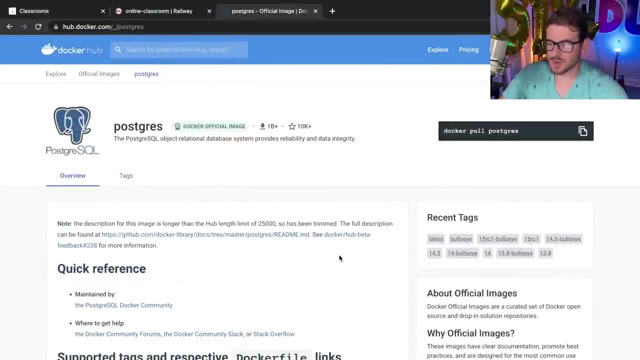 and you can basically specify what container you want to run or what image you want to run in your local environment. um, so in this case i'm saying image postgres, that's going to go to this postgres image, it's going to download it and then it's going to install it and it's going to uh run. 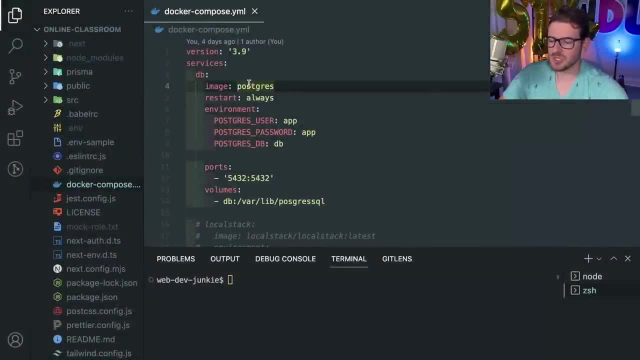 it- i shouldn't say install it basically just downloads the image and then it runs it on your machine, right? so it's going to run it and then it's going to install it, and then it's going to. let's show you that real quick. if i were to go ahead and just say docker hyphen compose. 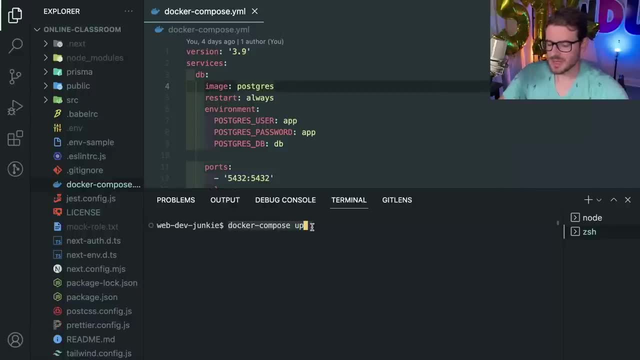 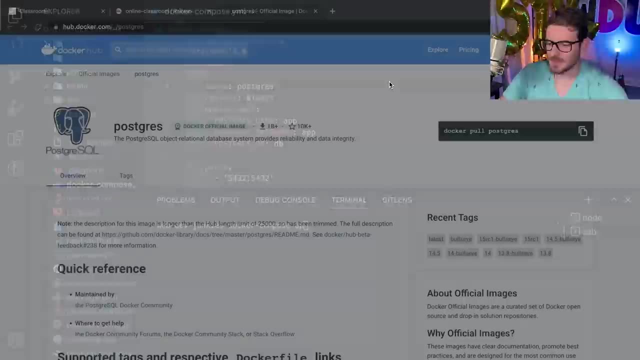 up now. granted, i think i have docker desktop installed, so if i go to docker desktop you will see an application load up, um, that basically shows all your containers. all right, so over here i have docker desktop set up on this laptop, which you can kind of like dive in and see. 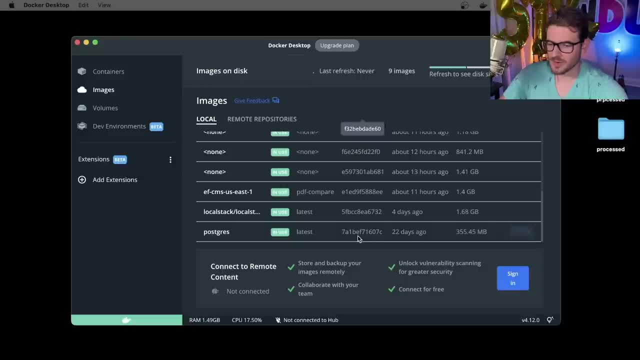 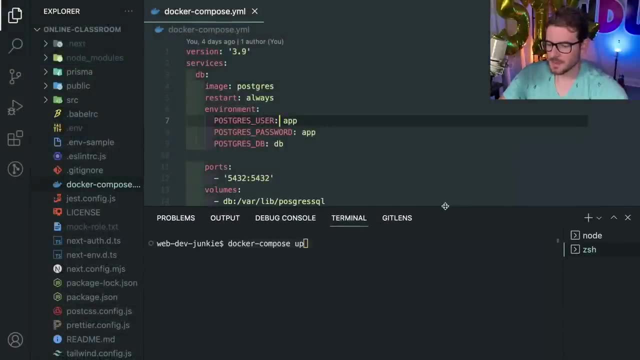 what containers are running and what images you've downloaded already. um, but when i do a docker compose up it's actually going to read through this docker compose file and docker compose is a separate. you know cli tool you have to install and you also have to have docker installed in your machine. but 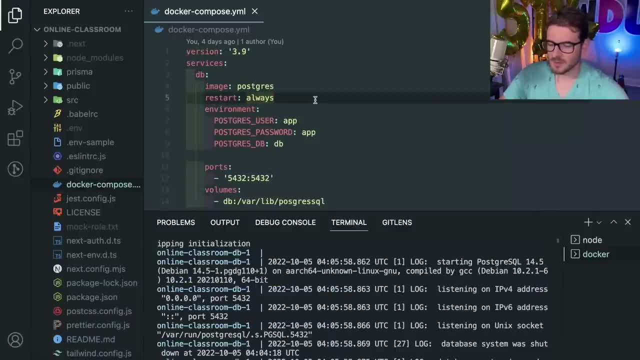 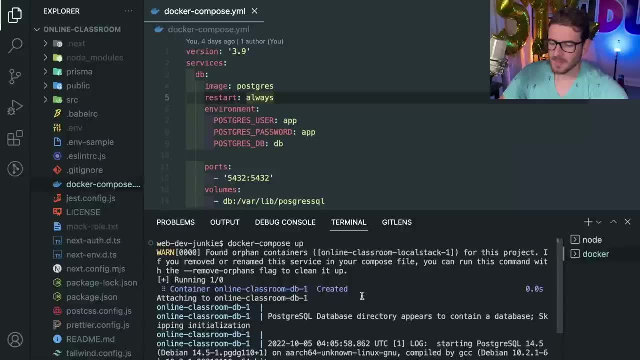 when i run this, it basically runs through this yaml file. um, if you're not familiar with the yaml, it's basically just like a more concise way to write json, without having all the curly braces and stuff. but it runs through this and it checks to see what services aka like what containers you 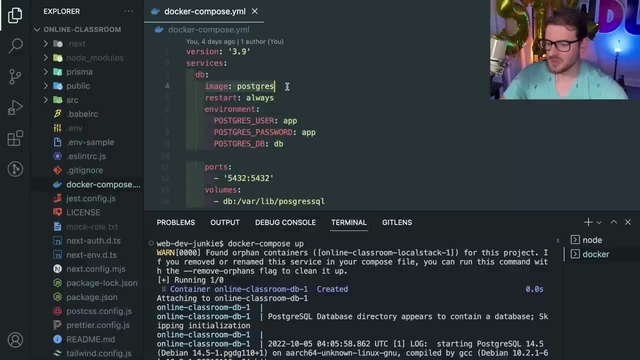 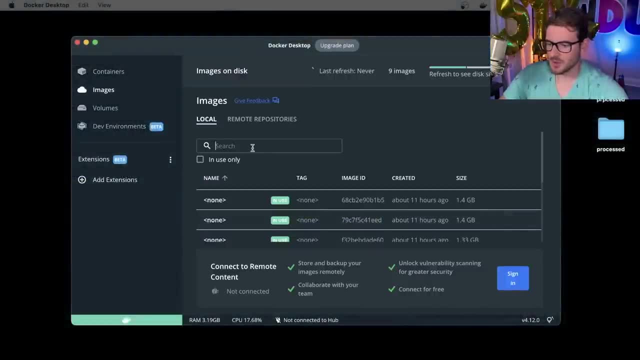 want to spin up. it looks at the image and it'll download the image to your machine if you don't already have it. so i'm assuming that if i go over to docker desktop, i should have an image over here that's called postgres. okay, so that's what got downloaded from the internet. it's about 355. 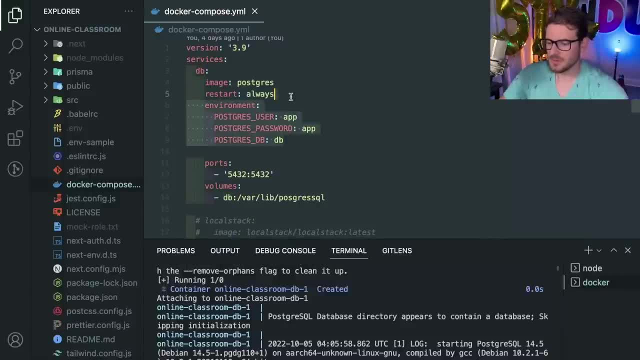 megabytes and once it's downloaded you can kind of configure it with environment variables. so i'm saying that these are the environment variables i'm going to run the container with. in this case i'm saying the user and password is app and app and the database is db, and i can actually kind 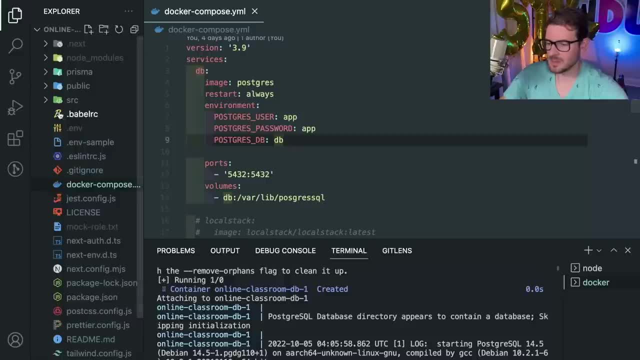 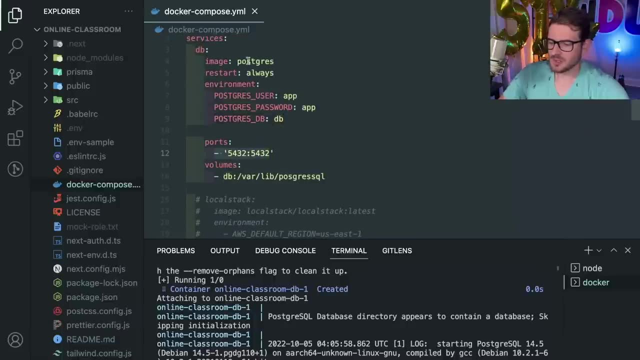 of connect to that locally using like pg, admin or any type of like vs code extension that supports that, and then you also specify like what ports you want this container to run on. um, in this case, i believe this is the host port and this would be inside the machine. so if i wanted to run this, 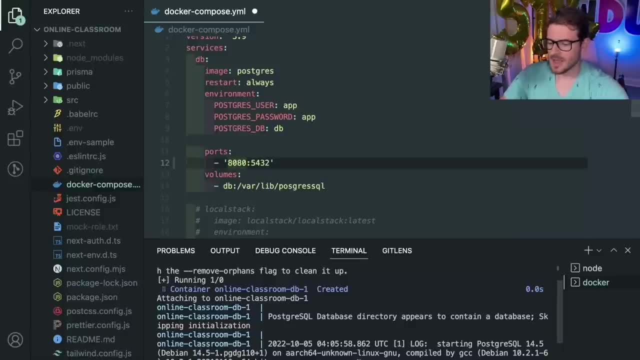 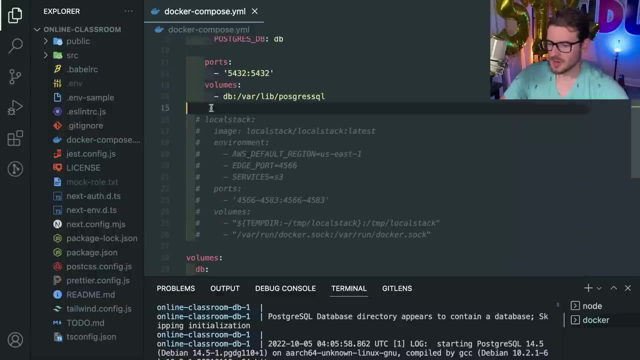 database on port like 8080 on my laptop, and then that would basically map my laptop's 8080 port to the internal docker containers. image of 5, 4, 3, 2 i believe. so that's how you do ports: you basically map your host to the actual machine. so if i look over here at a, i'm going to delete this. i don't. 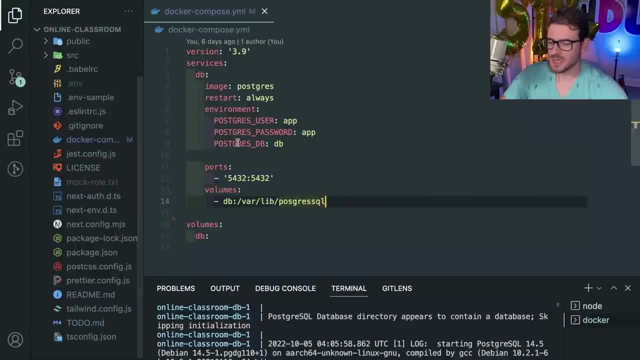 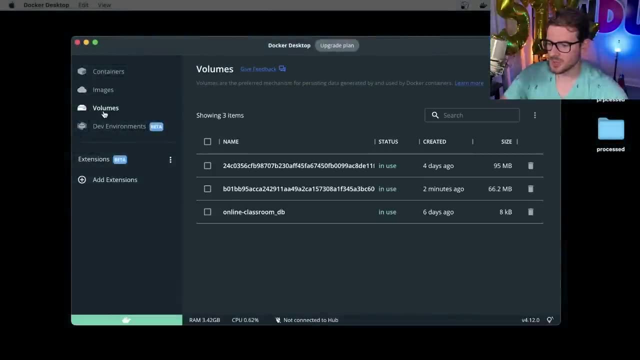 do that anymore. but look over here it's mounting a volume to the docker container as well. so this is pointing this db volume which is defined down here, and i believe docker desktop will kind of show you that volume, which will be probably called this one online classroom db and it's basically 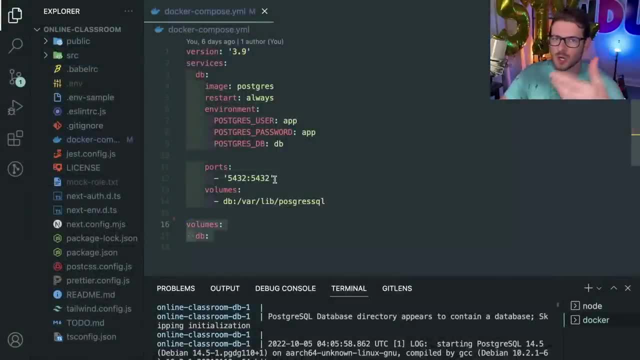 linking that, that volume, which is basically acts like a hard drive that you can attach to your container and it's saying: make this postgres service have access to this db volume and again it's going to show you that you can add this db name to a location inside of the container itself. 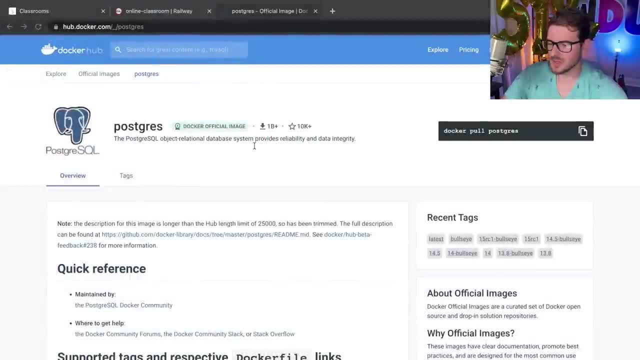 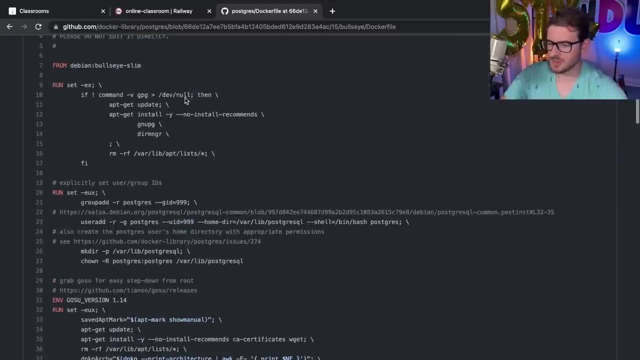 so it's kind of confusing if you don't really know much about docker, like you'd have to go and understand it. but all of these docker files- they're built up using just a bunch of like, basically some shell scripts, like you can actually dive in to see how the docker file was set up and 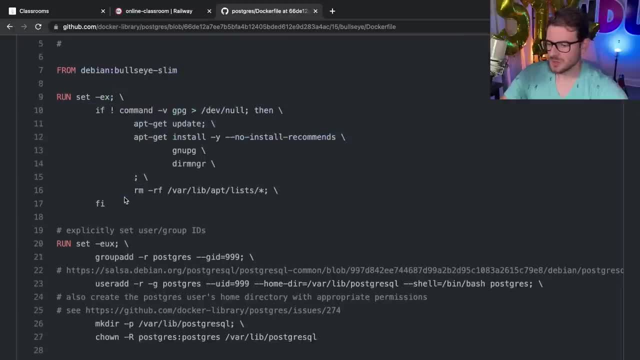 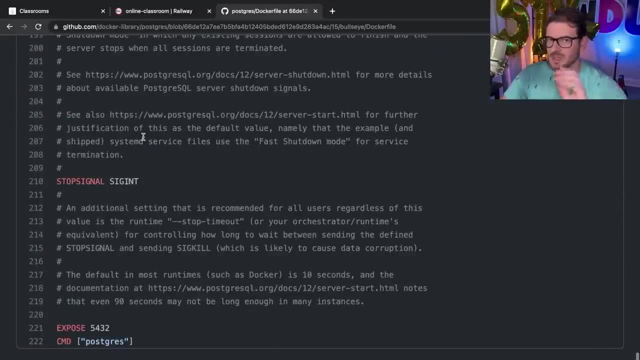 you'll see that it kind of decides what the base image to use and then it installs a bunch of stuff it might use like apt or apt-get to install and update after it does all these things. so it's kind of like this self-contained image that you can actually run up and have it run. 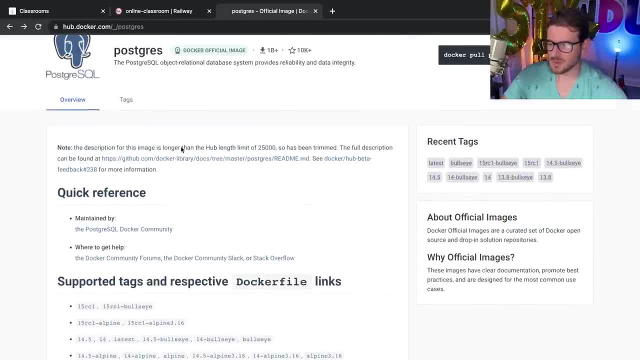 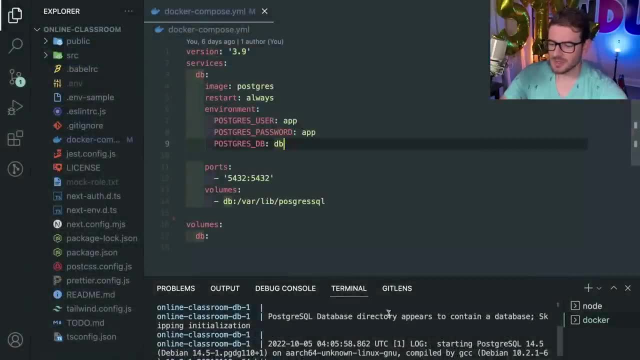 postgres or you know, you can do the same thing with mysql. if you're doing some other type of database, you can do that. there's, you know, open source docker images for all these different services. so the main purpose of all this is: i can have anyone clone this project. 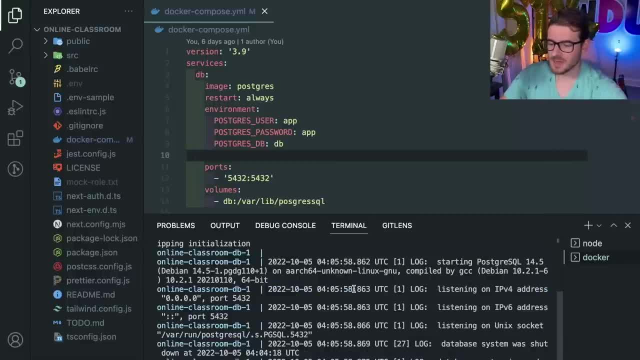 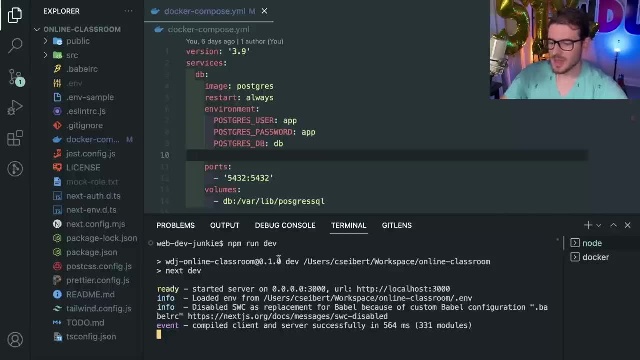 if they have docker set up in docker compose they can just run one command. they get a database going and then they could just go ahead and just run the service with an undev. and now they're good to go. they have a local running database. the service is already. 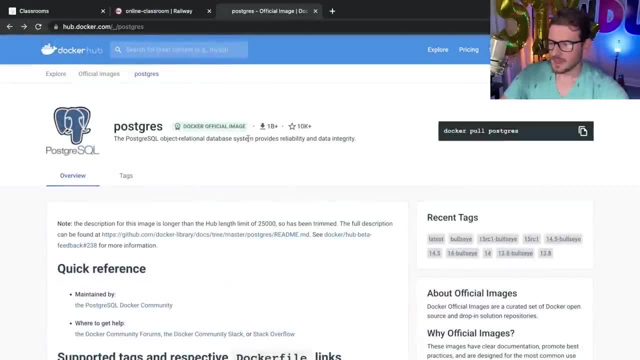 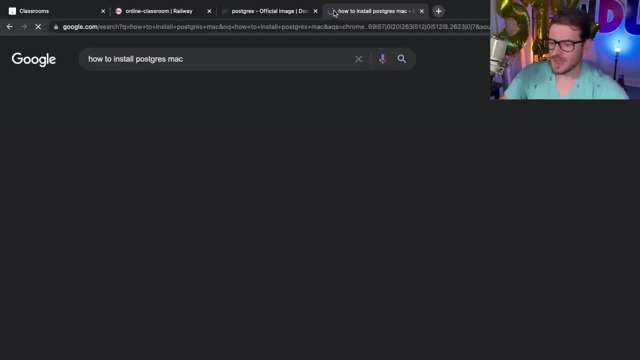 going to connect to it. um, and then they don't have to worry about doing any type of configuration because, like if you were to go and look up how to install postgres on mac, there's going to be some blog posts or some you know bunch of steps that you have to do. you might be able to brew. 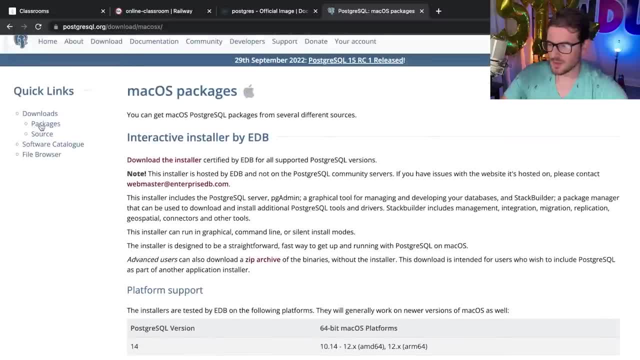 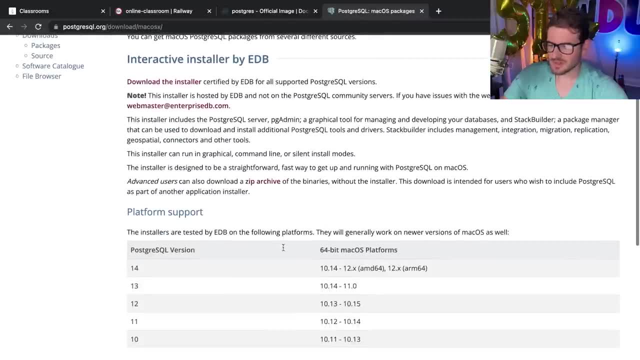 install it. you may not be able to brew install it. you may have to go and like find a package um for your operating system and then every os will have like a different set of steps you have to follow, and for a beginner it's just a real pain. 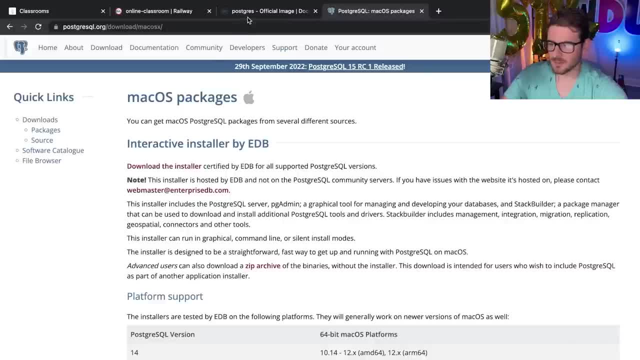 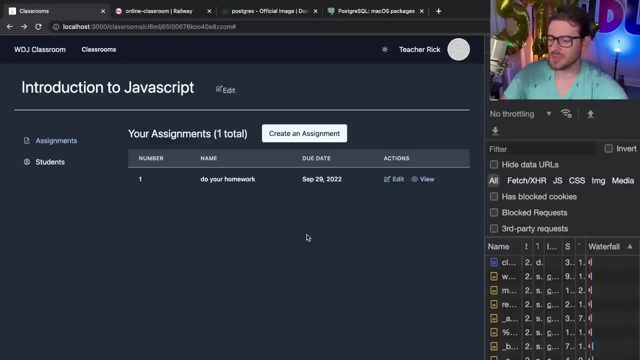 if you're more experienced, it's not that big of a deal to get these things installed. it might burn up 30 minutes or an hour of your time, but that's not stuff that you want to kind of waste your time on, especially when you're on a team of a bunch of developers and you want them all to have.